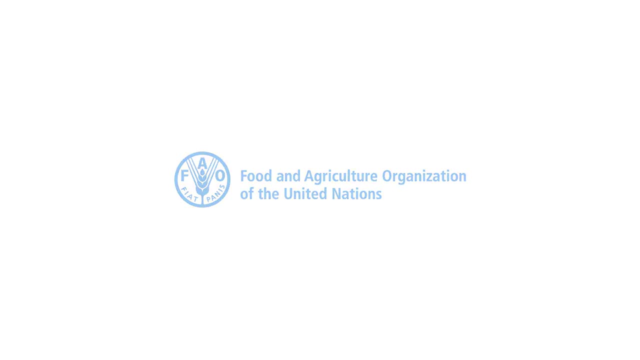 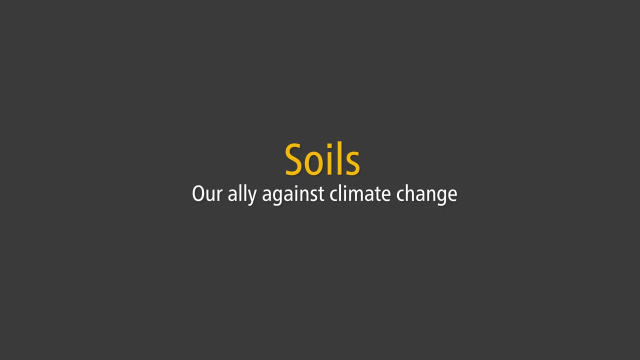 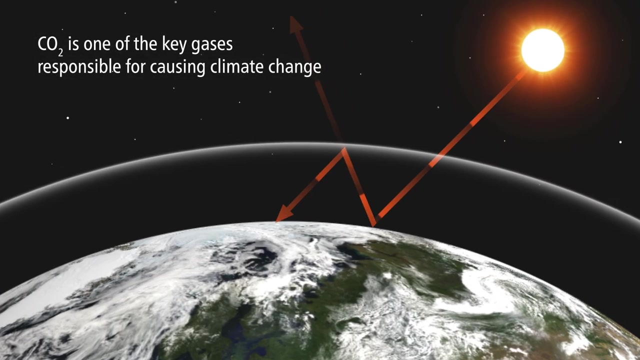 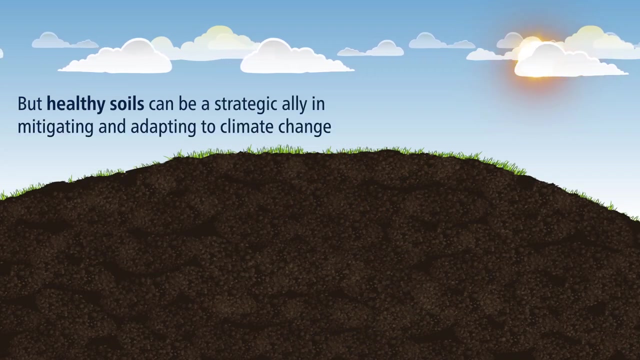 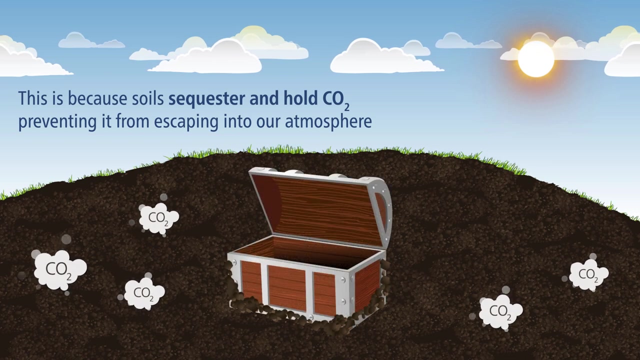 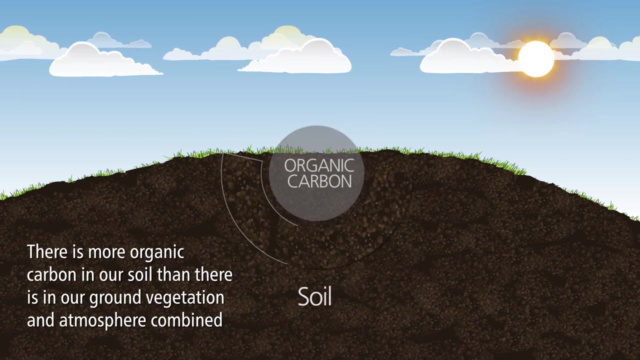 Carbon dioxide is one of the key gases responsible for causing climate change, But healthy soils can be a strategic ally in mitigating and adapting to climate change. This is because soils sequester and hold carbon dioxide, preventing it from escaping into our atmosphere. There is more organic carbon in our soil than there is in our ground vegetation and 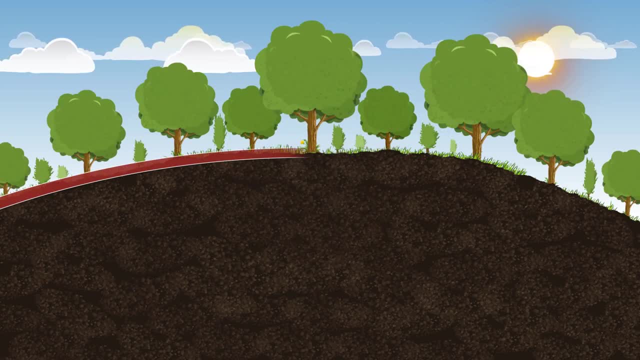 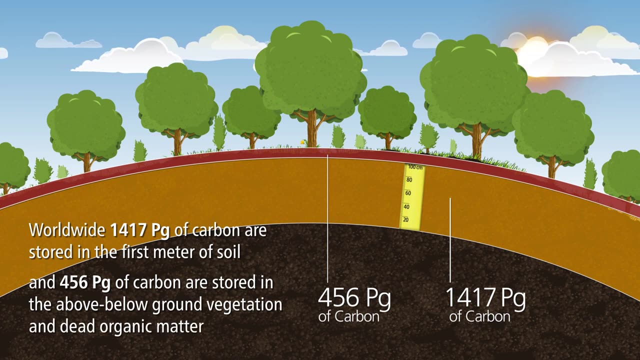 atmosphere combined. Worldwide, 1,417 petatons of carbon are stored in the first meter of the soil. 456 petatons of carbon are stored in the first meter of the soil, The above-below ground vegetation and dead organic matter. Organic matter plays a critical role in 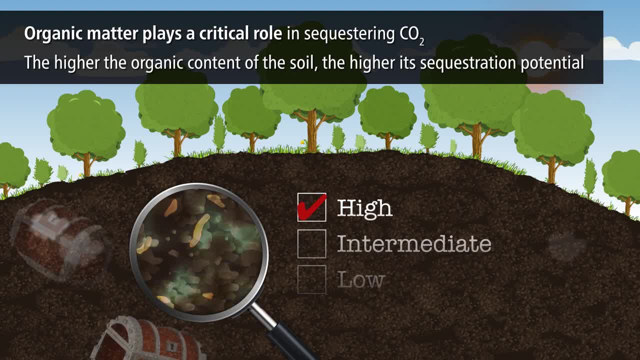 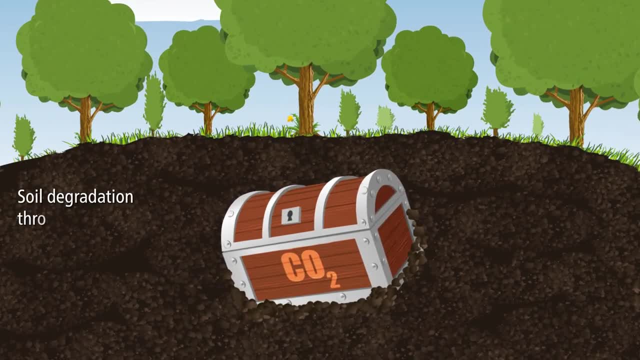 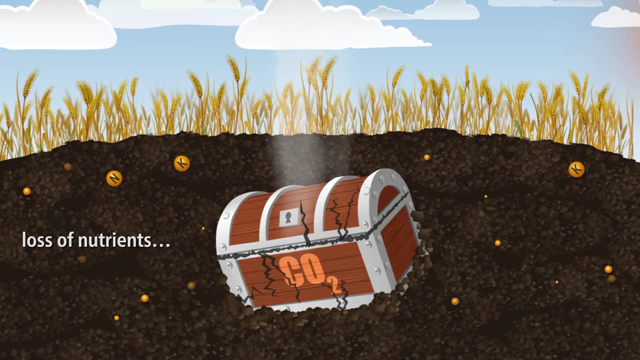 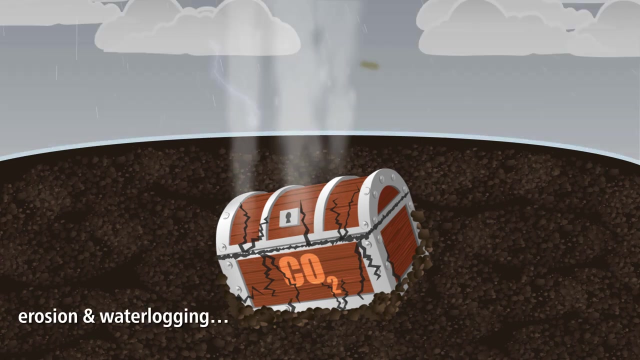 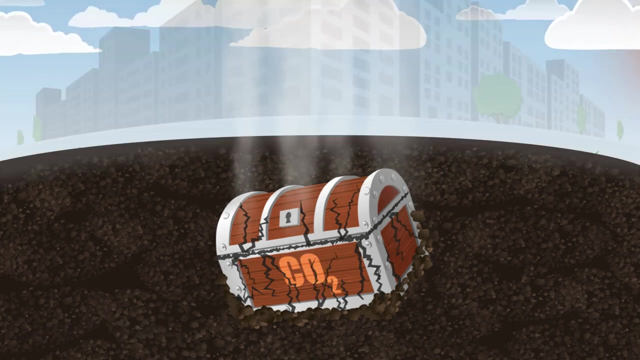 sequestering carbon dioxide. The higher the organic content of the soil, the higher its sequestration potential. However, soil degradation through deforestation, loss of nutrients, compaction, erosion and waterlogging and urbanization cause our soil to emit greenhouse gases that contribute to. 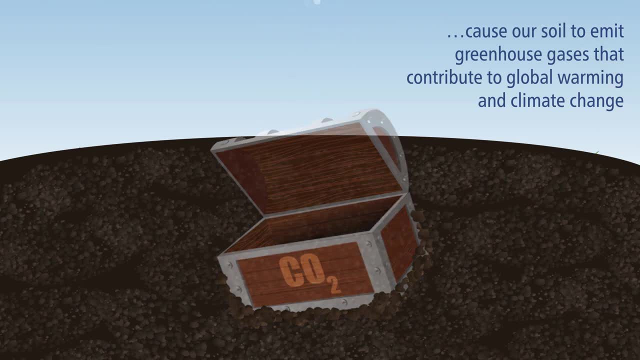 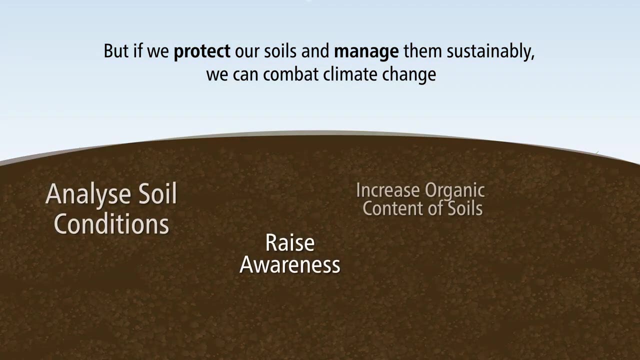 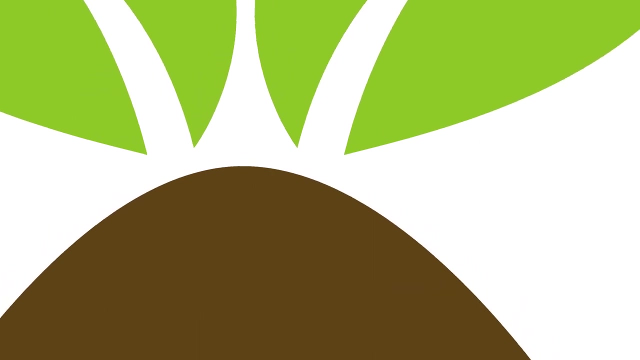 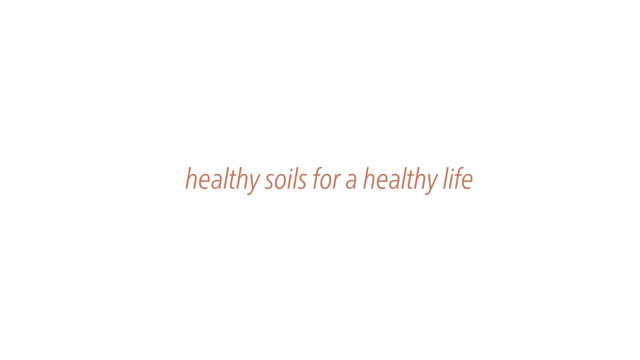